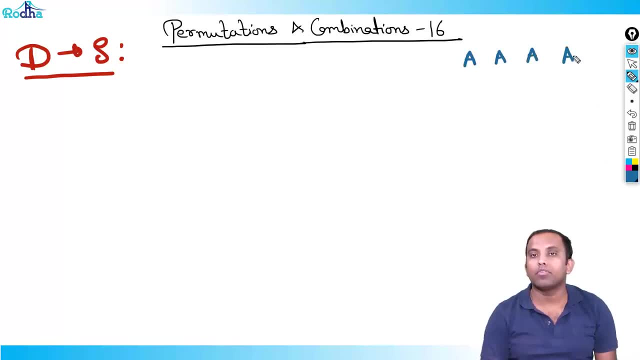 are four identical letters, double a. double suppose a, a, a. in how many ways you can select any two. Select any two. In how many ways? Only one way. Because there are four identical right Any two. you select only one way. You select first. second. you select first, third, you. 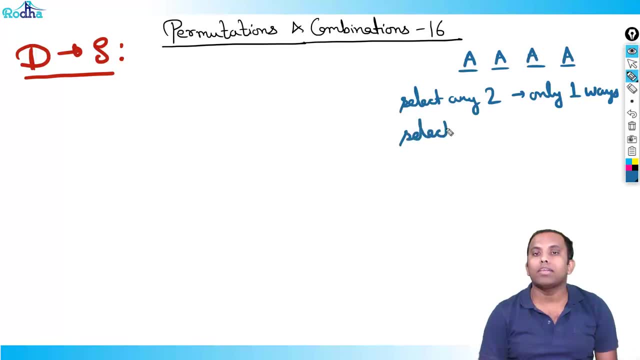 select second, fourth. all has to be only one way. In how many ways you can select any three? Only one way, Only one way, right? You select any three: first, second, third or second, third, fourth- all will look alike, right, Because all are identical. So out of. 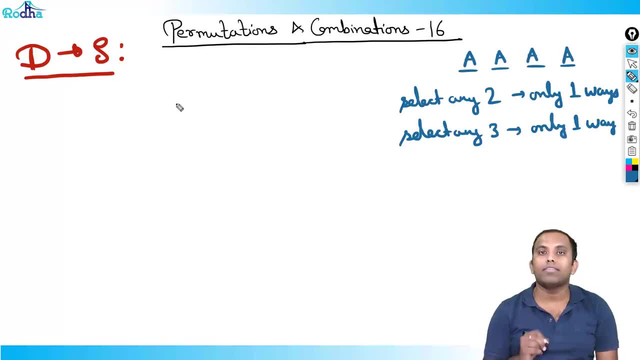 n n similar things. selecting r similar thing only one way right Out of n different thing. selecting r different thing ncr way, In this case, out of n similar thing. selecting r similar thing, r similar thing only one way right. r could be any of the value less than n. okay, So in this case. so we'll discuss. 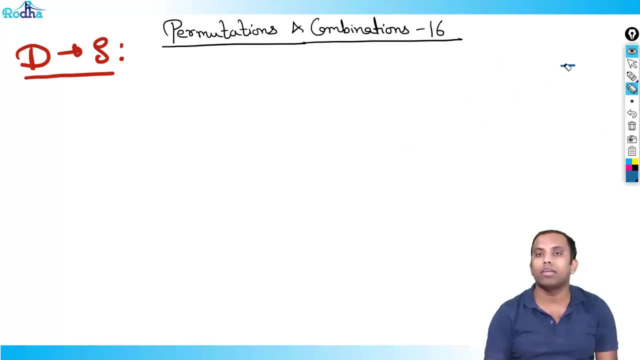 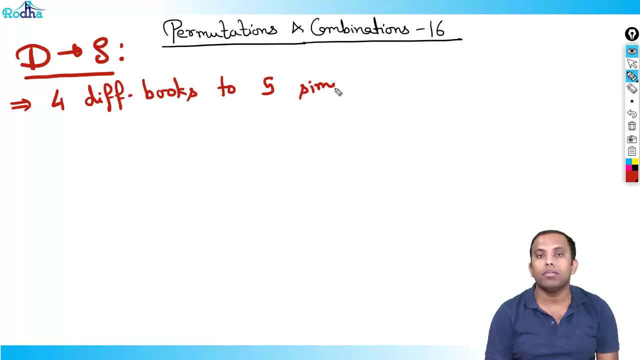 Now see, we'll do a lot of questions here, right? Different to similar to similar to similar. Then we can. we'll bring that equation to this context, right? How to solve by equations, How to solve by method, right? A lot of concepts are there in a few videos, right? Please watch. 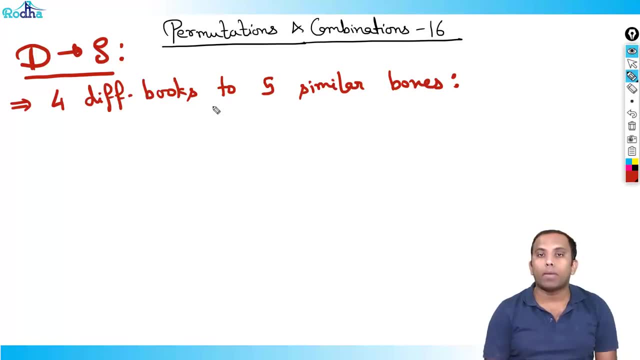 each video very carefully. So four different books to five similar boxes, similar boxes, right? Well, in this case I'm to put, let's say I've to put, there are five similar boxes, name it Like. all are like B, B, B B and B Right, All are identical, All are absolutely identical. 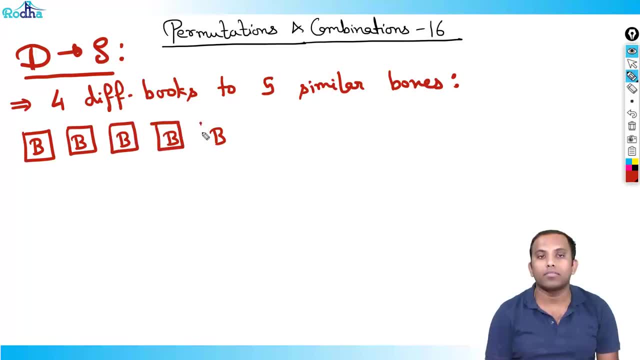 right? Similar in PNC means identical. You can't differentiate, right. There are five identical boxes. Okay, In this you have to put four different books like math, chemistry, physics, biology. So what we're going to do is we have to put them. in this case, 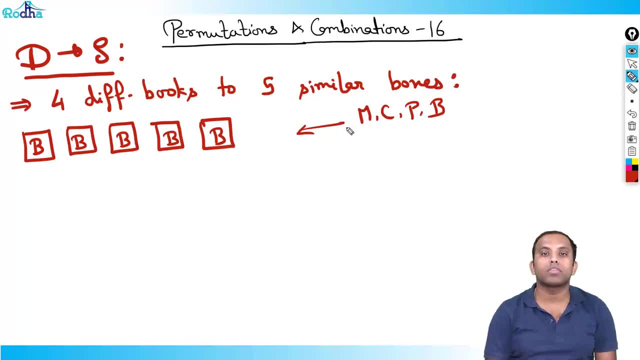 Okay, all are identical, right, All are identical. Alright, very simple, essential books. All are identical, existing in PNC, In this case physics, biology, right? So putting these four different books now in the in this I can't do. 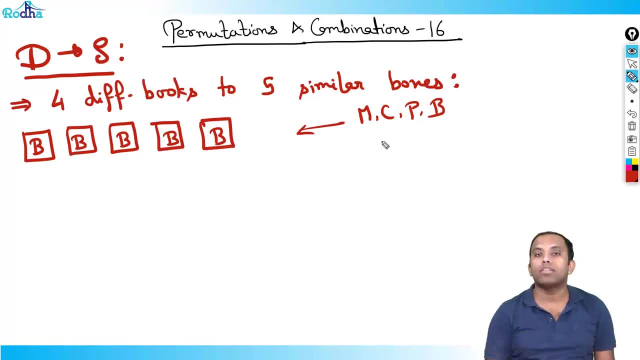 directly as a shortcut by circles and partitions, Because in this case, all these four books are different, right? So while selecting only this, there will be some cases. now. select any two- four- see two ways. select any three- four- see three ways, right, They're not identical. 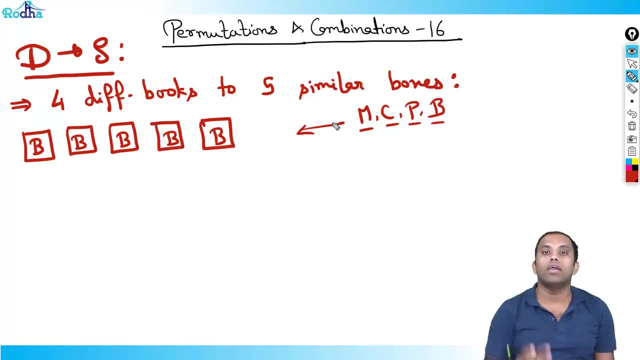 right, They are not identical. while selecting any three, only one way in identical. but here selecting a three is how many ways? for C, three ways, because all three are different, right? So there are five identical boxes. So how many cases I can form? So how many cases I can. 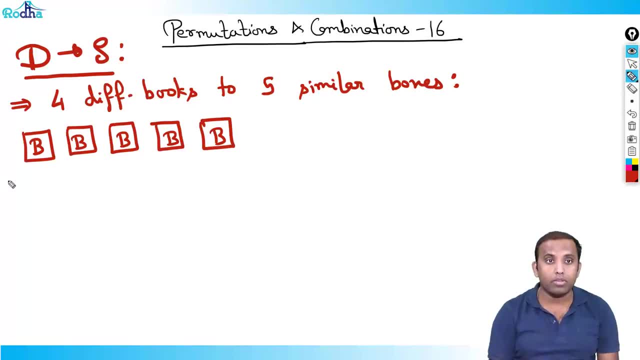 form here. So number of cases I can form here is how much? four different books. so for just make the cases here, how many cases for 00001 keys right. Three, one 001. these to one, 1000. one is two. to 00001 keys. 111101 keys right. these are the five cases. 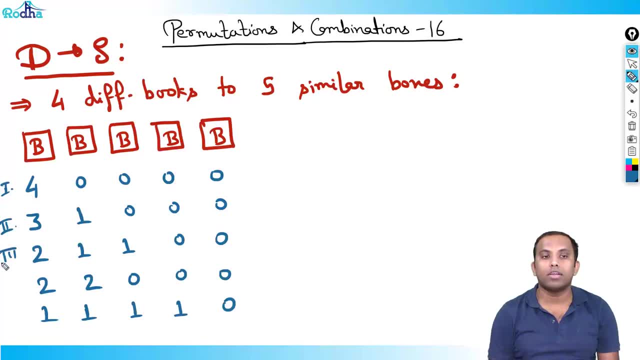 I can make first case, second case, third case, fourth case and fifth case. right, Jayramientic, five cases I can make now. Now distribution: right now there are four different books here, So let's say they are maths, chemistry, physics and biology. So how many ways in first? 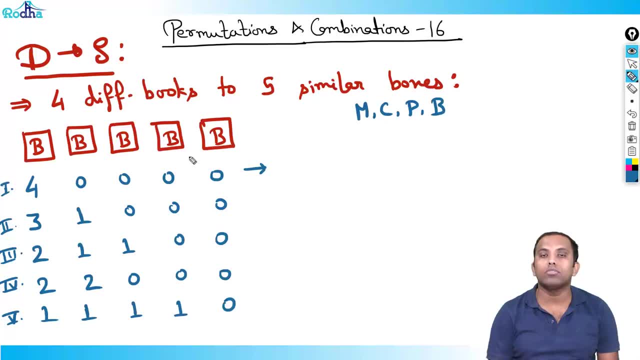 case, how many ways you can put this four books as 400000.. So 400000 here means see all these five boxes. all these five boxes are absolutely identical, are absolutely identical, right? That means, if you put four boxes in one box and you close that box, right, So you have. 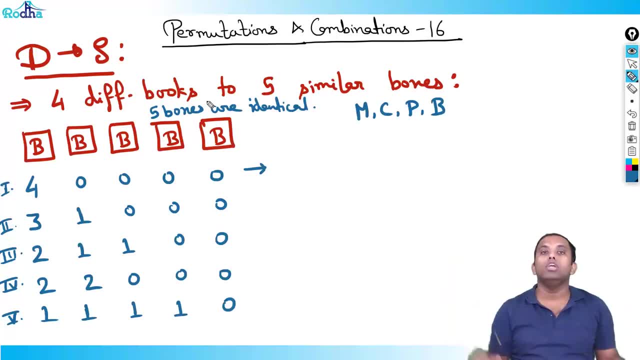 still five boxes in front of you, five identical boxes. you don't know in which box there are those four books, Right? So no any nonsense questions here like okay, I know which in which box I kept, or what if I keep the boxes open? right, I listen this kind of answers. 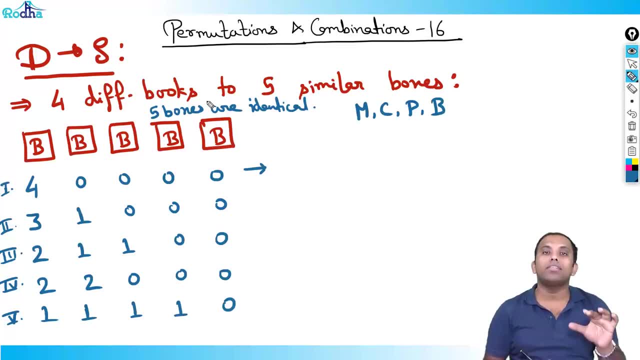 in the class, right? So don't think like that. in P and C, Similar things means absolutely identical things. Okay, so four different boxes are there. Okay, sorry, five of five similar boxes are there? Five identical? that means five identical boxes. boxes are there. 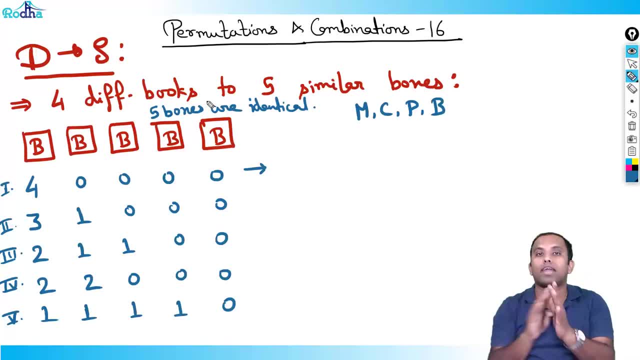 So in which box there are four books, in which box there are zero books? that cannot be differentiated, right. That's why we will not do shuffling shuffling when we will do when we are different, when we are different numbers, which we have to put two different, different variables right. 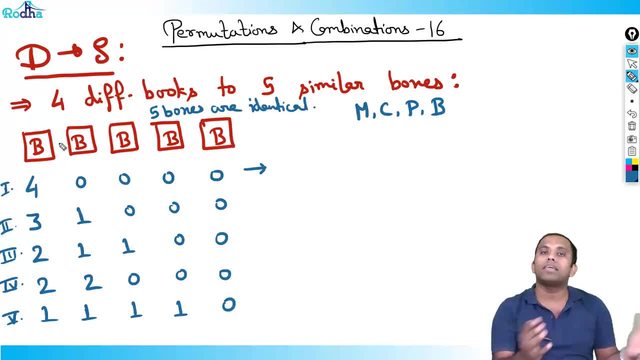 there we do shuffling, Here I don't need shuffling because all five are same right. So here, out of four books, selecting any four is how many ways? 4C4.. What is 4C4?? One 4C4. 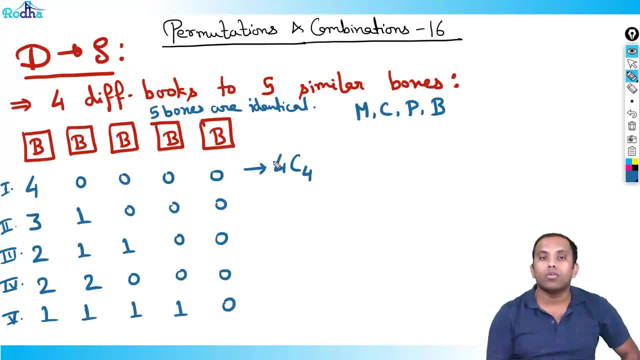 is one right. Four books are there. selecting any four: only one way. Now, putting in any of these five boxes, only one way. Okay, selecting in 4C4 ways. putting in any of these four boxes: only one way, right, because you can't differentiate between the boxes. Okay, so 4C4 into one is. 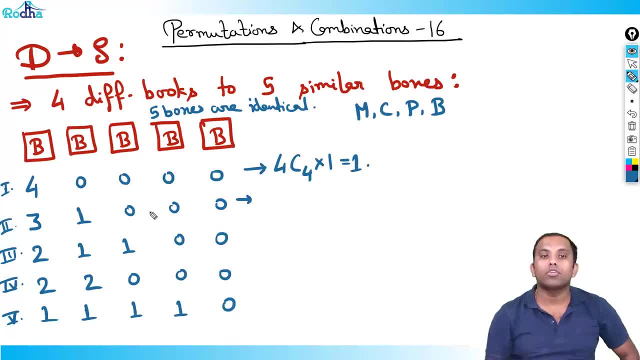 one, Fine, Second one: 3100.. Now here the five, two will come right, Because out of four books you need to select three books. Now, which three books? right, This can be done in how many ways? 4C3 ways, Out of four books selecting. 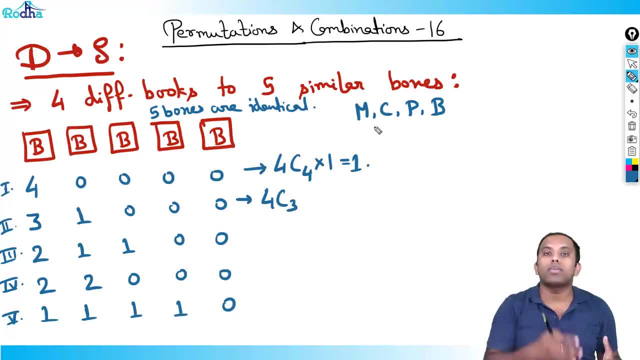 three books, right. So how many groups of 3-3 I can make, How many groups of 3-3 books I can make? 4C3 group: What are those? 4C3 group: 4C3 equal to 4C1.. 4C1 is equal to. 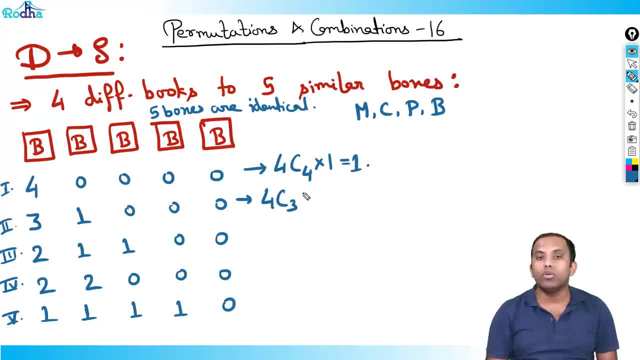 four. Okay, Now, that means now, see, don't think anything else here, Once, I suppose, out of this. So 3-1 case, 3-1 case, right, When you select any three book. that was Maths, Chemistry. 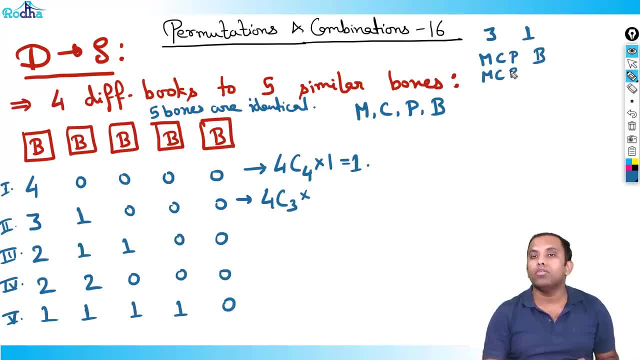 Physics, Bio is left, right. When you select Maths, Chemistry, Bio, Physics is left. When you select Chemistry, Bio, Maths, Physics is left. Okay, sorry, All these two are same. only When you select Maths, Bio and Physics, Chemistry is left, And when you select Physics. 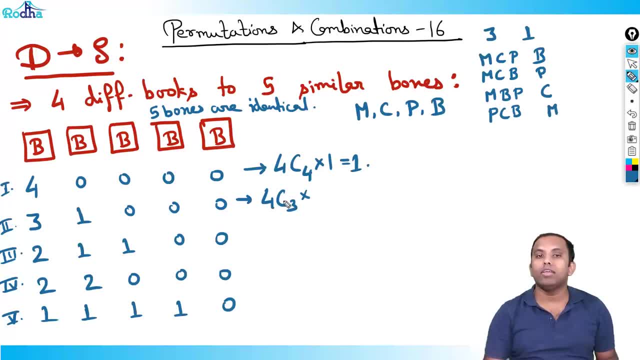 Chemistry, Bio Maths is left. These are the four cases: 3-1.. 4C3, that is equal to 4C1,, that is equal to 4.. These are the four cases right Now. that means now in one hand. 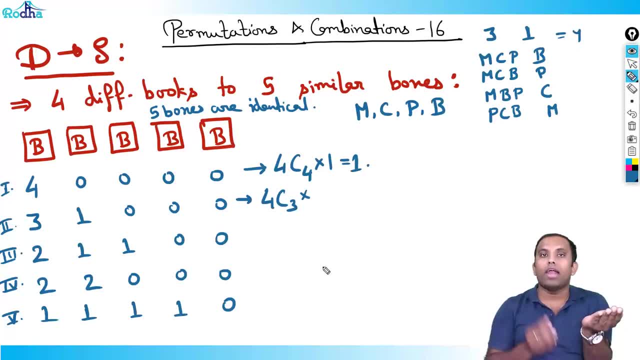 you have three books, three books which are selected, And the other hand you have one book, right, So two groups now, one book of three, group three, one group of three book and one of one book, right? So in one hand you pick three books, In one hand you pick. 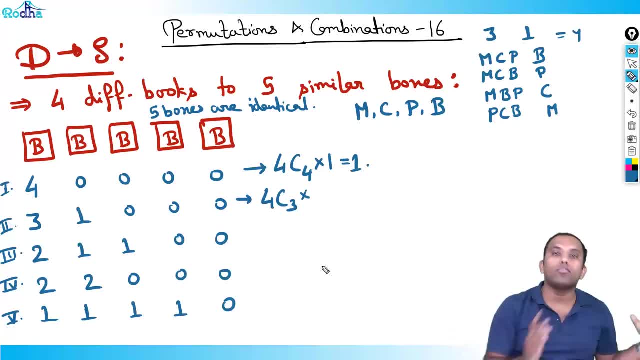 one book, both the groups. okay, you put in any of the boxes, it doesn't matter, Right? It doesn't matter, right? So 4C3 for these four cases, selecting any one book, it doesn't matter, It's already. 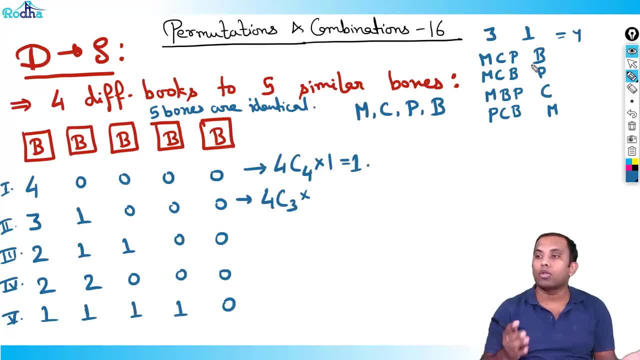 groups are formed now: 3 and 1.. When you pick three: automatically one is left right. There are no, there's nothing, any, anything. there's no way else for forming any group right. When you're out of four books, you select three, automatically one is left. So 4C3 into. 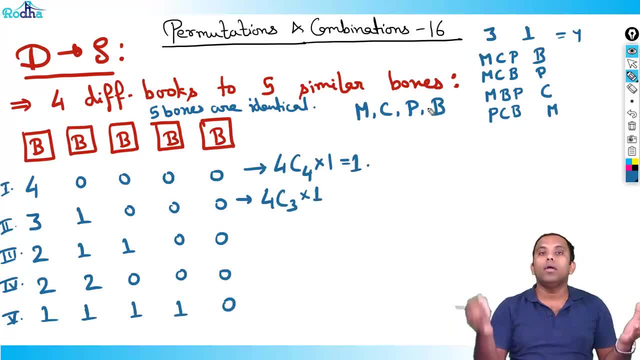 one. Selecting this one book, only one way, Okay. And putting this 3 and 1, two groups in any of the boxes, only one way, Right, Because in one book hand you have three books, In one hand you have one book. 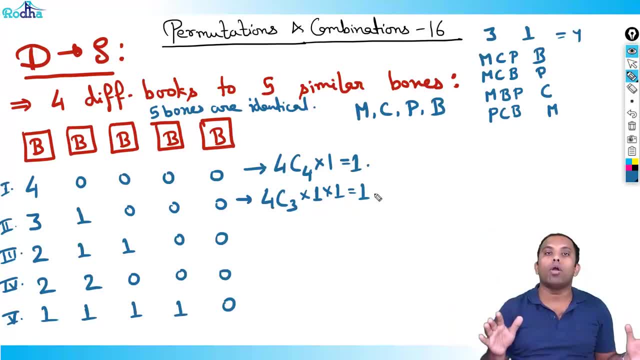 You put in any of these two boxes, it doesn't matter, because all these five boxes are identical. It doesn't matter, right? So what is the answer? Sorry, 4C3 into 1 into 1,. what is the answer? 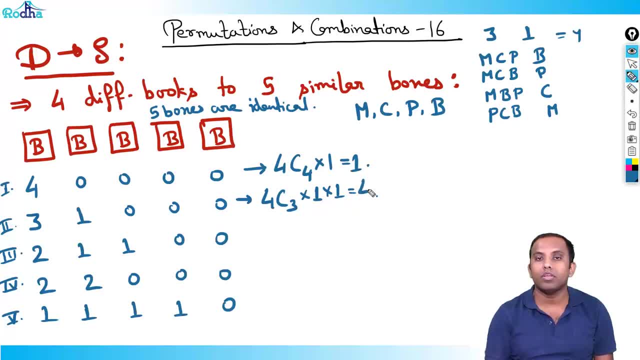 The answer is 4.. So answer is 4 here. Okay. Now third one: 2, 1, 1.. Okay, 2, 1, 1.. Okay, then just 2, 1, 1.. Again, out of four books, which two will come? Okay, So 2, 1, 1, 2, 1,. 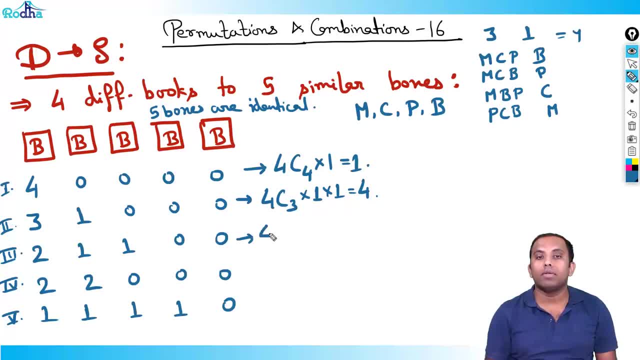 out of four books, which two will come. Okay, So that can be done in 4C2 ways. So out of four books, which two can be taken. That can be done in 4C2 ways. right, So out of four, 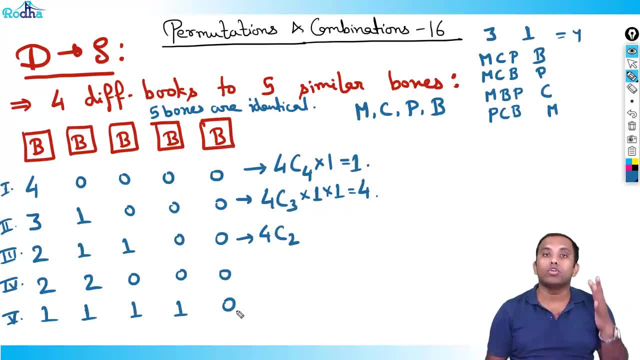 books, selecting any two in 4C2 ways. that means there are 4C2 groups. What is 4C2? Six. There are six groups of 2, 2 books. How many are left? 1, 1, right. Now you see this. 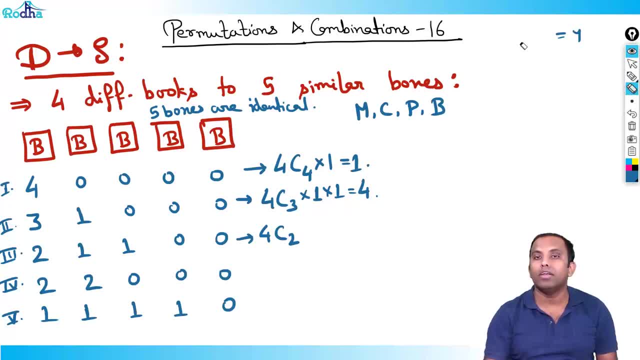 case now: 1, 1 are left, 1, 1 are left right. So once you make a group of 2, 1, 1 here, 2, 1, 1,- you select Maths and Physics. Bio and Chemistry are left. Select Chemistry. 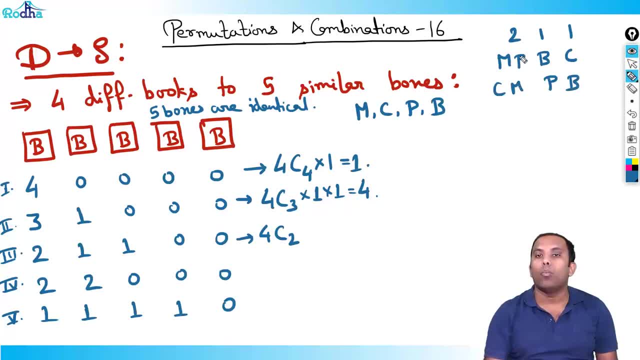 and Maths, Physics and Bio are left right. That means once you select these two books right. So you have to select. you have to make two groups of 1, 1 book. You have to make two groups of 1, 1 book right Once you select these two books, like Maths and 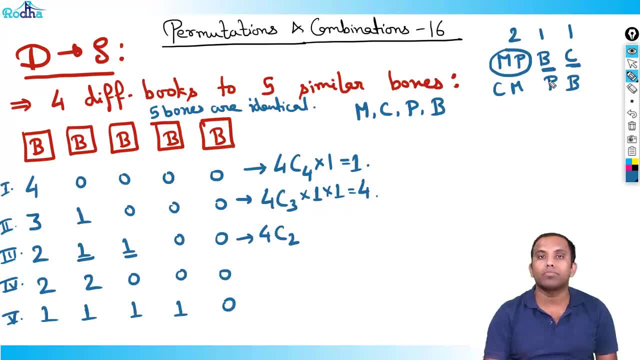 Physics. so you have to select two books for 1, 1 group. Okay, So either way, right? You don't have any option to select because you have in one hand. you have 2, 2, 1, 1, 2, 1,. 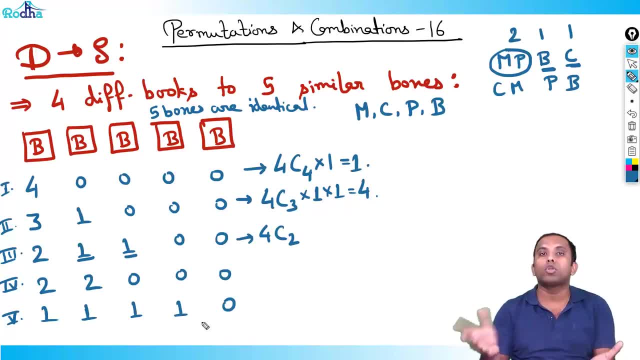 you have two books and other way you have two books, you have to make group of 1, 1.. So in each group only one book will go. So no other option of making any group right. So 2, 1, 1, you select any. understand this thing right. When you select two books, two 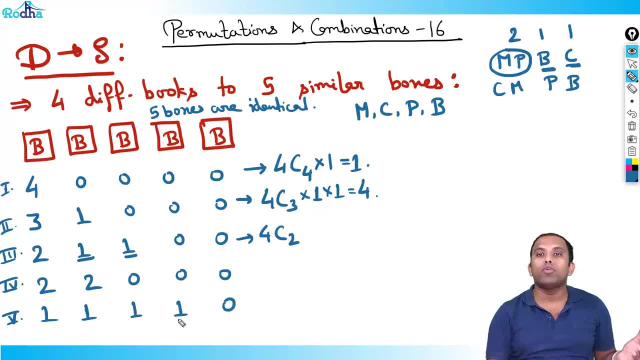 books are left Out. of those two books you have to make group of how much? 1, 1. So there are no option of selecting right In either of the group. only 1, 1 book will be there. 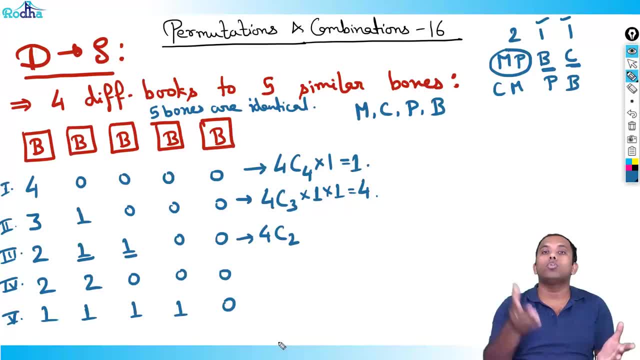 Why it is it, it, it. it won't make any difference, because that group of 1,, 1,, 1, 1 will be put in any of the boxes in only one way, because all the boxes are what They. 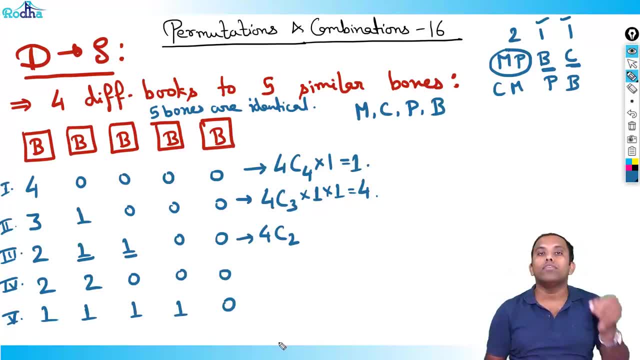 are identical. So absolutely no difference, right? So once you select, once you select those two books, okay, then two books are left. Two books: you have to make a group of what? 1, 1.. So in one group there will be only one book, right, And that putting. 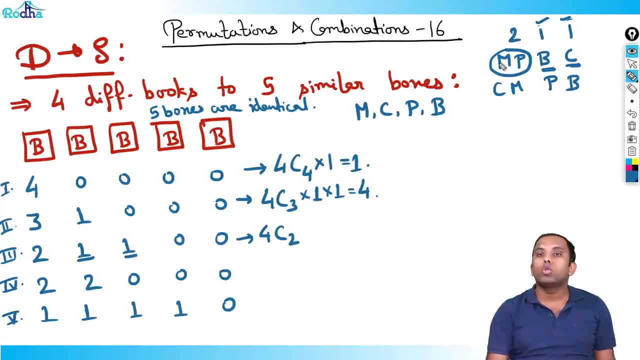 will make no difference in the boxes, right? Only one way. That's why two books are there and two groups are there. So two groups of 1, 1 book are there. So there's no option of shuffling right, Because both the ultimately they have to be kept in boxes and all the 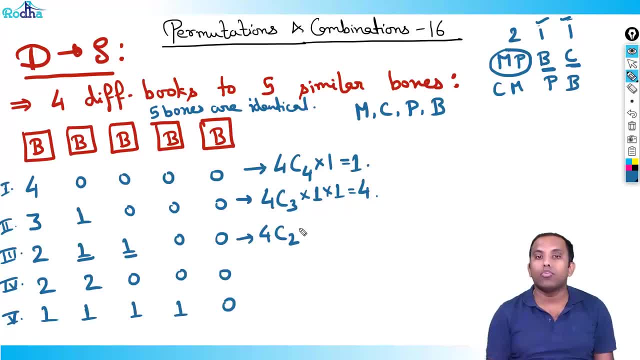 boxes are identical, So no difference, right? Therefore, 4C2, now for this two group: two books and two. two group of 1, 1, only one way of making right. And putting these three groups of 2, 1 and 1 in any of the three boxes will not make any difference, only one way. 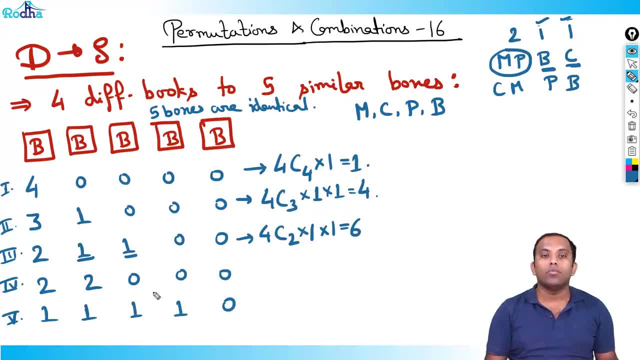 It is again 6,, again 6, right Now. we'll discuss this case in the last part of this video. Thank you for watching Now. let's discuss this case now. I told you, if there are two books and you have to make, 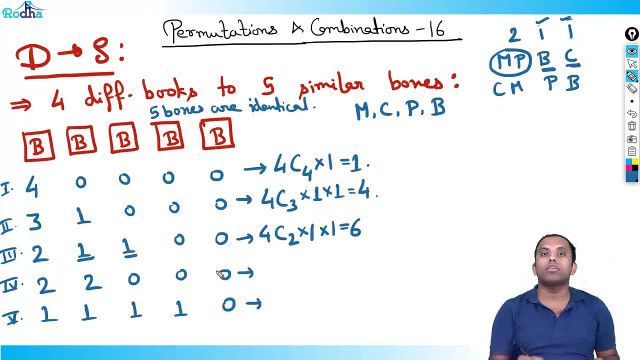 two group of 1, 1 book. there has to be only one way right, Because there's no option of selecting Same way here. What is the answer for fifth case? There are four books and you have to make four groups of 1, 1, 1, 1.. So only one way right: Four groups, and you have 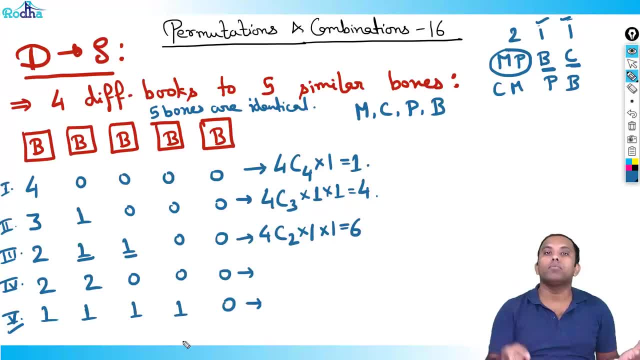 to make four group of 1, 1,, 1, 1.. Only one way, because in one group you can pick, you can keep only one book. In one group you can keep, you can keep, you can keep you. 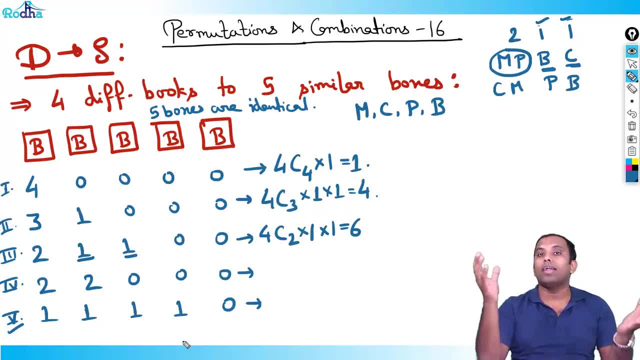 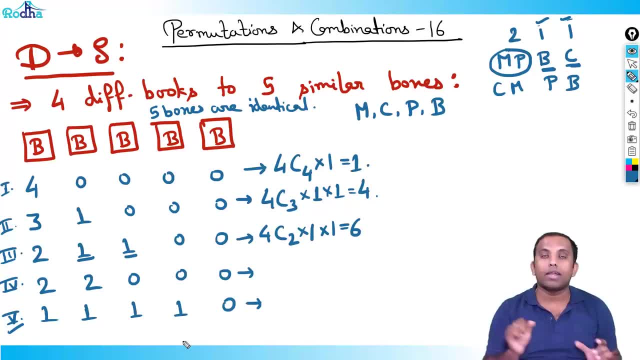 here 1, 1, 1, 1, 0.. Fifth case: That means there are four different books here: Maths, physics, biochemistry. So out of four different books you have to make four groups of 1,. 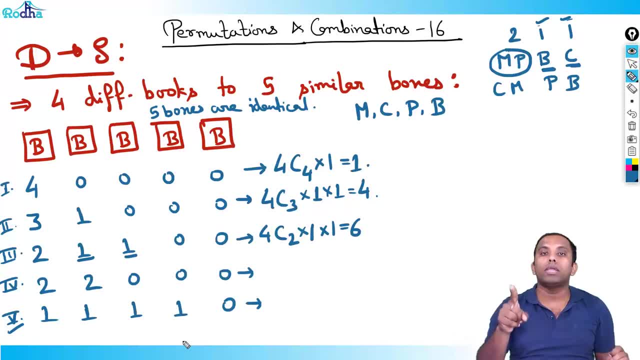 1, 1, 1 book. Okay, In one group you have to keep only one book, No option of selecting right. So there are four groups of 1111 book. you can put those 1111 book in any of these boxes. 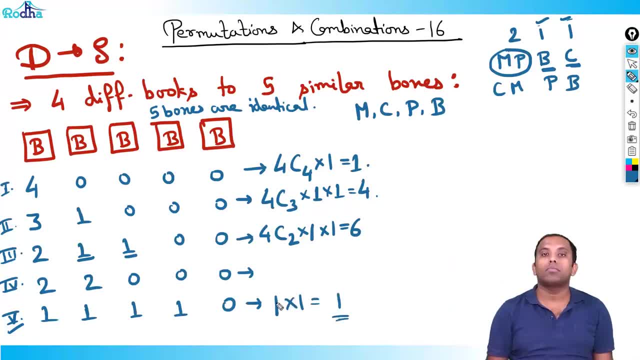 only one way, Right, So there has to be only one into one. So very nice concept, Right? If there are three books and you have to make three groups of 1111 book, only one way. There are two groups, you have to make two groups of 1111 book, only one way. 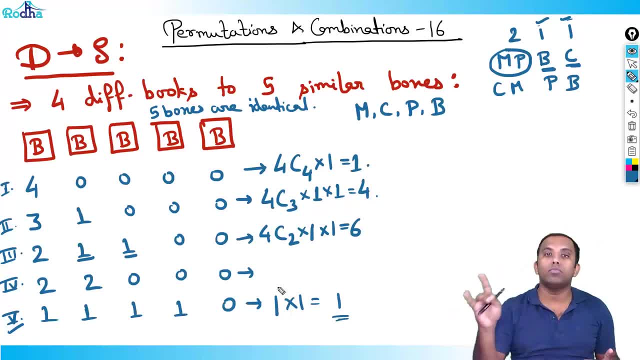 If there are four books, you have to make four groups of 1111 book. only one way, Right, Because you have no option of selecting. One group has to contain only one book and ultimately you have to put in boxes that are only one way, because all boxes are identical. 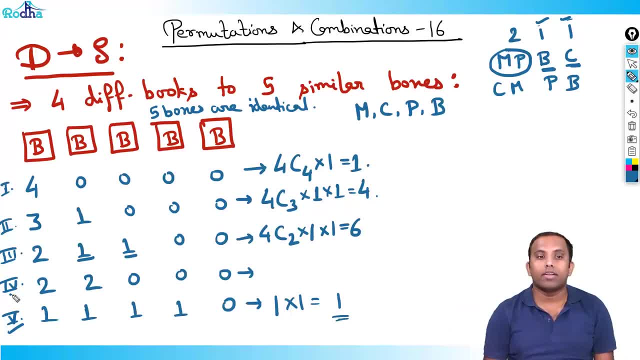 Now this case- fourth case here, right, this is important- case 2 and 2, this is important case here, Right, Normally, by what way we studied till now what we should do is out of four books we. 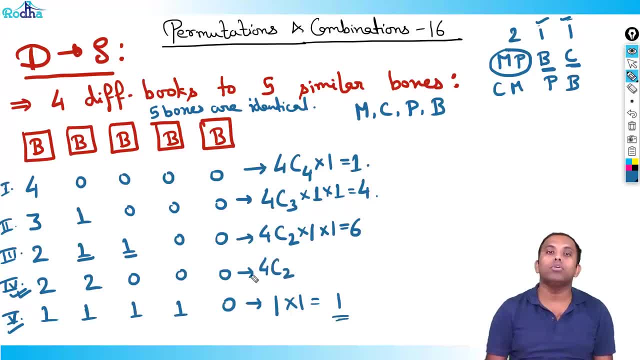 can select any two books in four C2 ways out of four books. we can select any two books in four C2 ways Right Out of in total four C2 ways. now two books are left. That's what I told. 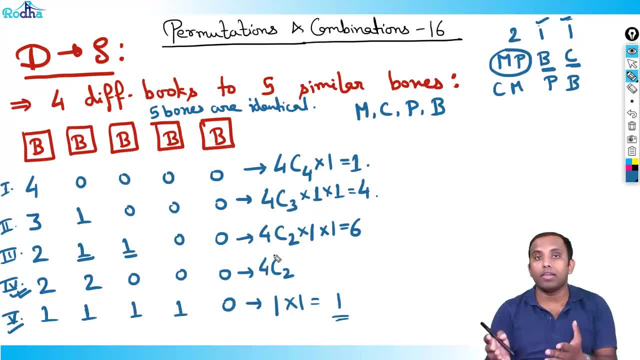 Right. Two books are left. There is no option of selecting. You can pick any two books and put in any of the boxes. only one way, Right. But here is a little bit of twist. See, we'll discuss that twist here. 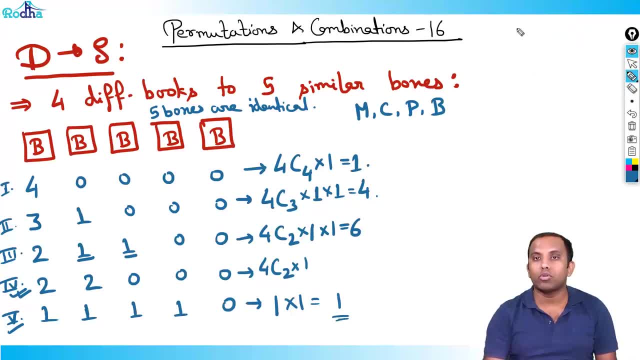 This is a case of 2-2. Right, This is a case of 2-2.. Books are Maths, Chemistry, Physics, Biology- Right. When you pick Maths and Chemistry, Physics, Biology are left. When you pick Maths and Physics, Chemistry, Biology are left. 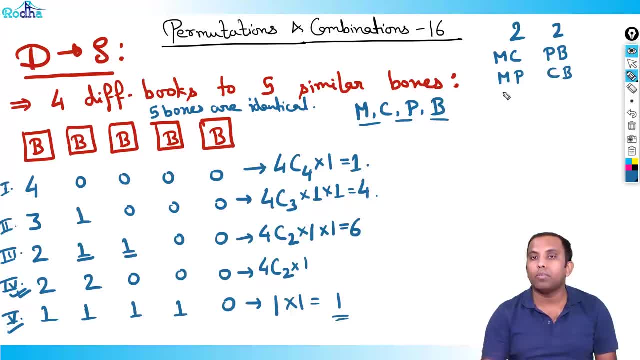 Right When you pick Maths and Biology: Physics- Chemistry are left. Right When you pick Maths and Biology: Physics- Chemistry are left Right Now, when you pick Physics and Biology, Maths- Chemistry are left. When you pick Chemistry and Biology, Maths- Physics are left. 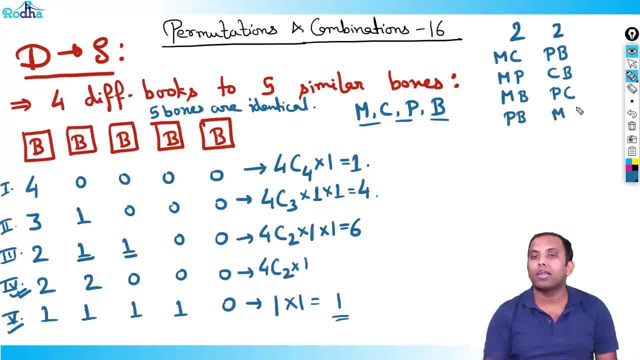 When you pick Physics and Biology, Maths, Bio are left, Right. These are your six. If you would say four C2, so four C2 means six. These are your six cases: One, two, three, four, five, six. 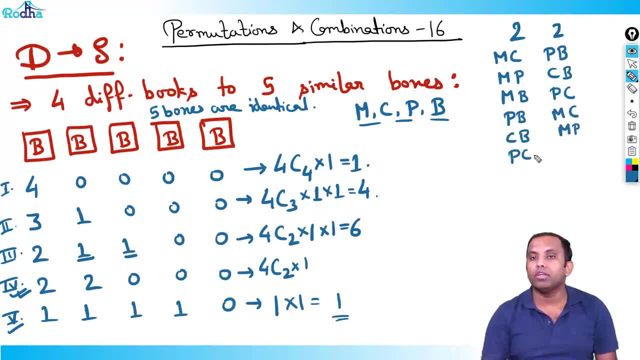 But you observe Because, since these boxes are identical, these are your six cases: One, two, three, four, five, six. But you observe Because, since these boxes are identical, these are your six cases: One, two, three, four, five, six. 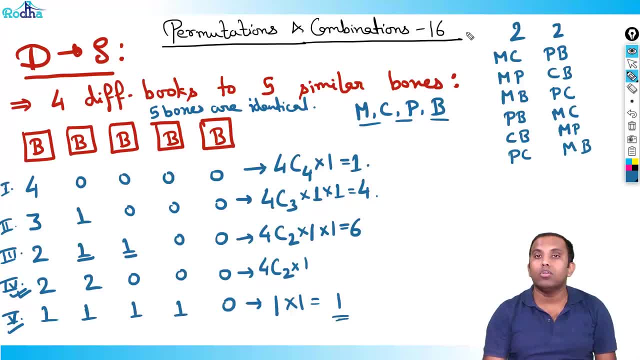 But you observe, these are your six. if you would say four c two, so four c two means six. these are your six cases: one, two, three, four, five, six. but you observe, because since these boxes are identical, so mass chemistry and phase bio, like this, and mass chemistry, physics bio, like this, these two are absolutely same. 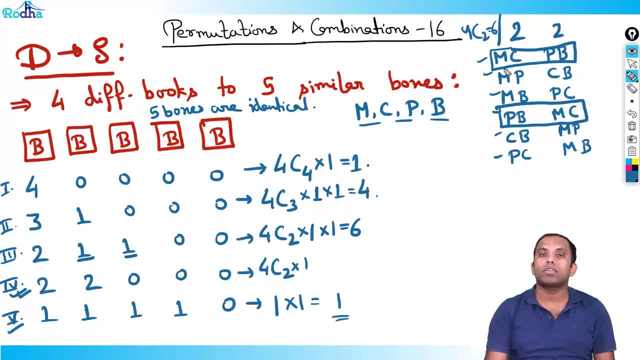 because in the flicks, in the first block it is mass chemistry and in second box it is mass physics, bio. and its reverse case is what? in the first case it is phase bio, in second case mass chemistry. right, all are same, only all are same. so absolutely no difference. right, because boxes are identical. so 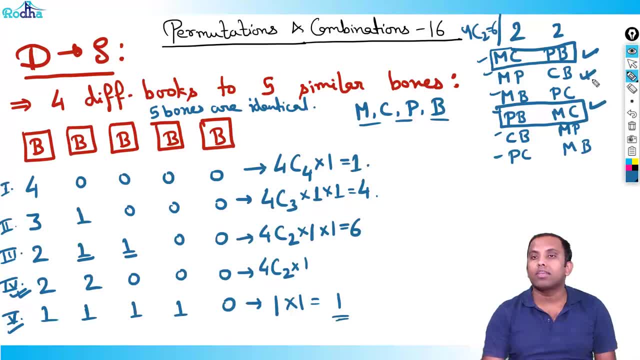 every two cases. see, this case is equal to this case here. this case is equal to this case- mass physics, chemistry, bio. and this case is equal to this case. right, so all these three cases are same. okay, that means there are not six cases, there are actually only three cases. 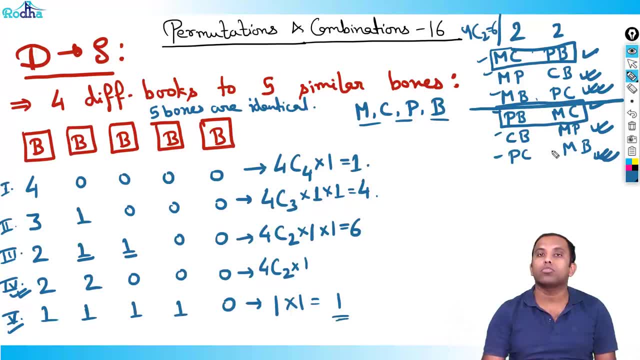 because first three case is equal to next three cases, because box is being identical. so it won't make any difference if first book, first box, has mass chemistry and second box has phoenix bio, or first box has phoenix bio and second box has mass chemistry- right, mass chemistry, same. 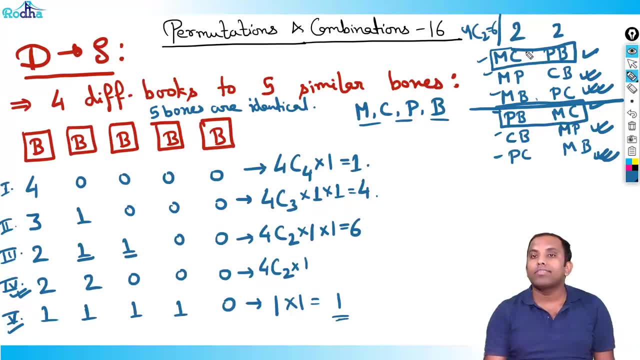 same thing. so how many ways? there are six ways. right, there are six ways, but six by two. so four c two divided by two. this is very important, funda, right, very important funda. here we're discussing four c two divided by two and placing this two, two group in only one way, that is three. 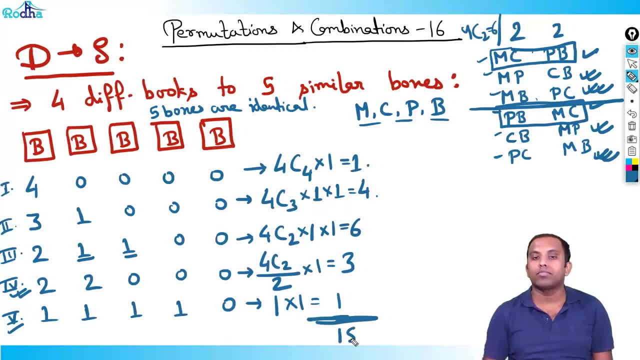 right. so what is the answer here? answer for this question is 15. answer for this question is 15.. right, this is the way to solve this case of different to similar right. in first go, it will look difficult. right, it will look difficult. of course, it's a very nice concept. 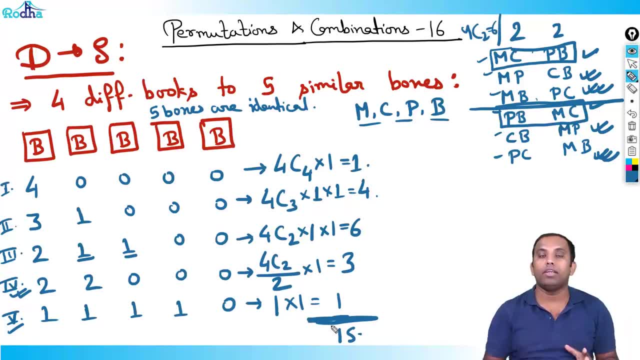 right, but don't escape from it. face it right. i'll, i'll give my 200 percent in explaining these things right and i pick these tough things right. i want to explain, i want to teach you these things right and you should learn these things to maintain your aptitude level, to develop your attitude level right. so maintain an attitude. 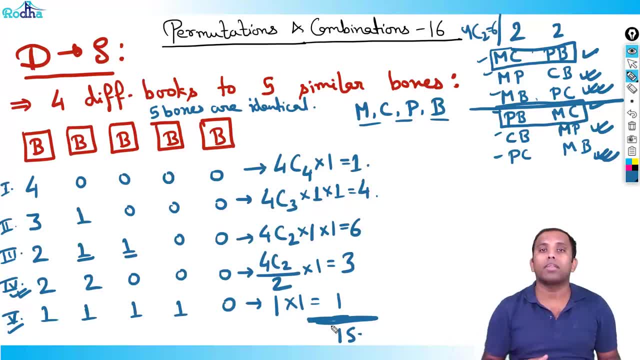 toward these things. right, you have to learn it. we'll do several examples, right, there's no limit of examples, right, but you have to learn this thing, okay. so this is the crunch point in all this, uh, in this whole question, is this part, this fourth one? so see, whenever this two and two are repeating, right, always, whenever this. 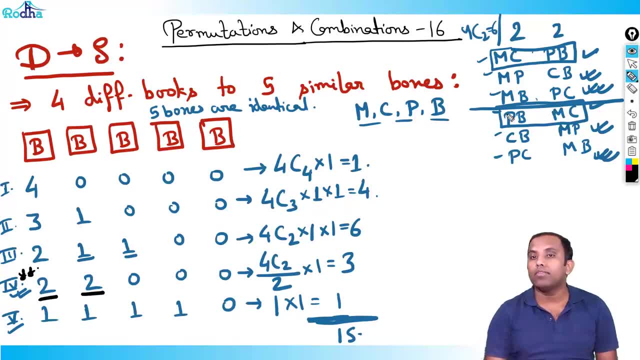 two and two are repeating because it will be, because it will be always in i, always there is symmetry between two and two. right, first two and next two are same. right because boxes will identical. right. so whenever you see any other number repeating, any number repeating other than one, because one repeat won't make any difference, because one box. 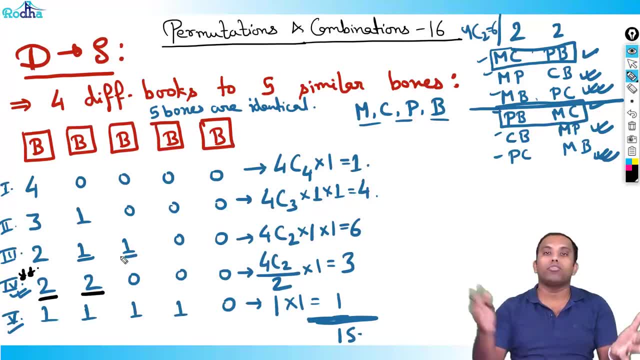 book is only one group, no symmetry. one in math, one in physics. no symmetry, right. but what? where is the symmetry with two, with two, right? with mass chemistry, phase, bio, phase, bio, mass chemistry, right. so this is symmetry, right? so whenever there's a other number, when, whenever there's a number, 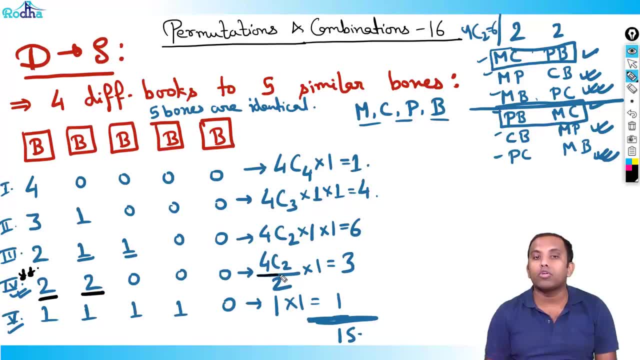 repeating other than two, always divide by two. because i could show you this? because there are only four c to six cases here, so i could write those six cases here and i could show you that these six are not six, they're only three. actually, first three and last three are same right. but if 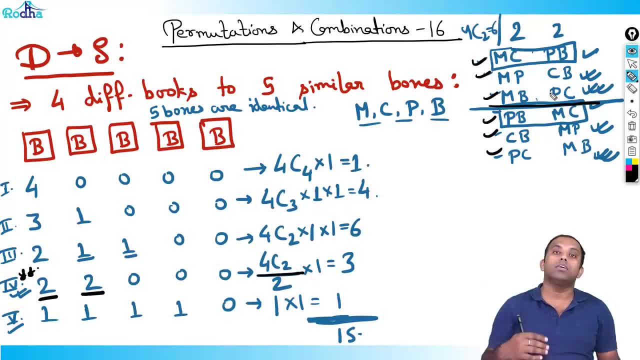 there are 30 cases. even i can't show you, or neither, or you also can't write those 30 cases, right? where is symmetry? where is the symmetry? so, whenever two is repeating two times, or any number other than two is repeating other than one is repeating, always divide by two, because there will be. 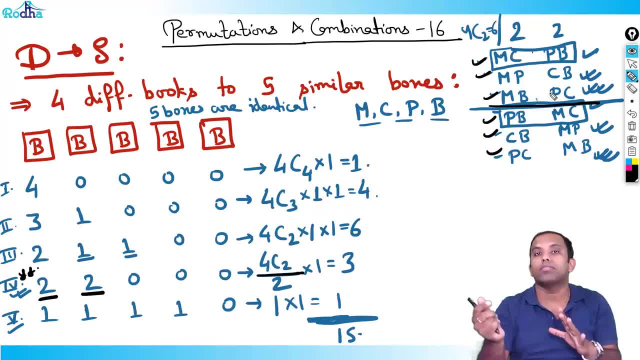 symmetry and when boxes are identical, that symmetrical case is equal. one, two and two one are equal if the boxes are identical. right, so always have. this case is very important. right, always has. this case is very important. so the answer for this question is: what? 15, in how many k ways four different books can be distributed to. 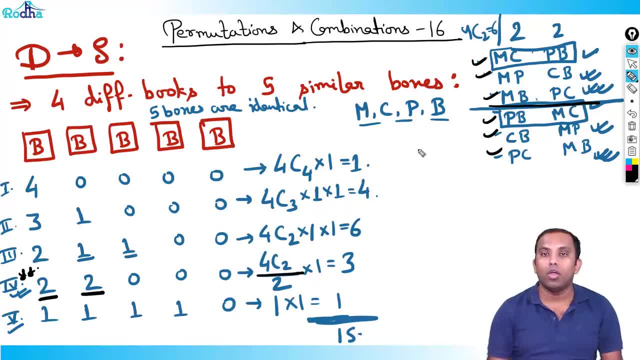 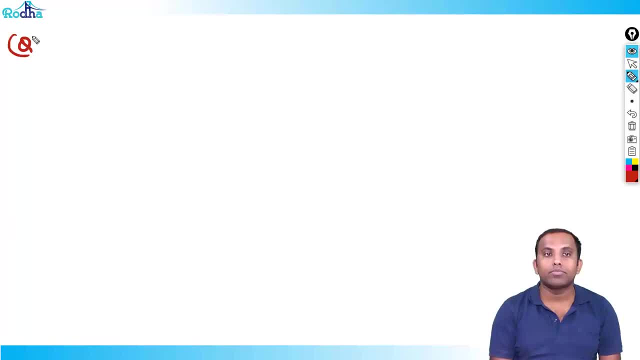 five similar boxes. what is the answer? answer is 15. okay, one more question we'll do on this concept: different to similar: okay. five different books to three similar boxes- okay, now don't leave the question exam if you face the exam. okay. five similar balls to three different. 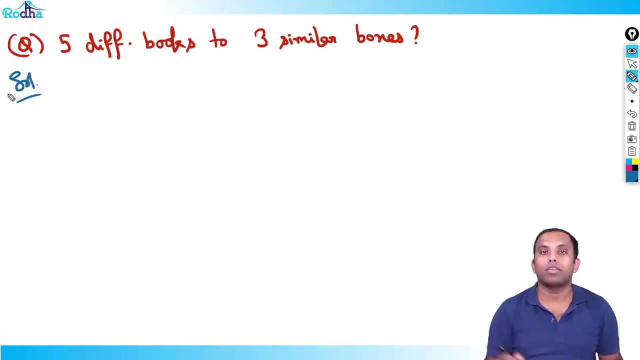 bags, you'll tell sir, only taught for books and boxes. right, so getting it right, assembly, it is what is the criteria, it is what it is: different to similar, different to similar right. so for all the cases where distribution is from different to similar, you can apply this funda quite easily. 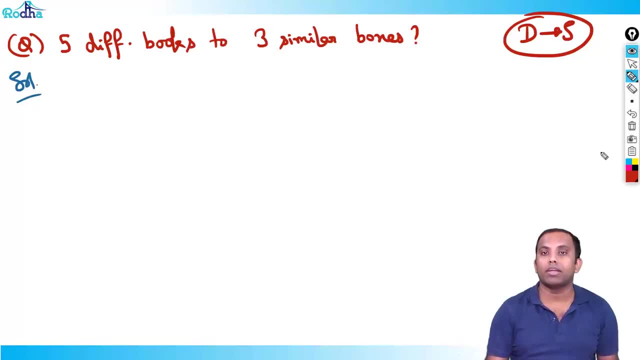 okay. so five different books to three similar boxes. right, again, we'll make this three boxes. we'll make this cases, make this three boxes and make this cases. three identical boxes, right, how many cases here? five books. so five zero, zero, okay. four one zero three, two zero three, one one. 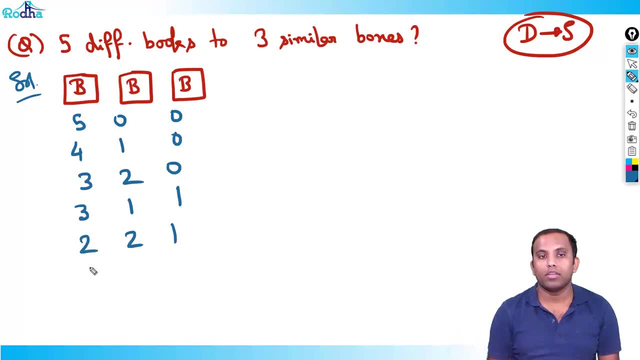 two, two, one, anything else, two, three, zero. okay, done three, two zero, three, one, one, two, two, one. good, we don't have to shuffle right, because again, boxes, boxes are identical, so doesn't five zero zero is same as zero zero five. okay, so these are the four cases, i think. yeah, fine, just five cases, five. 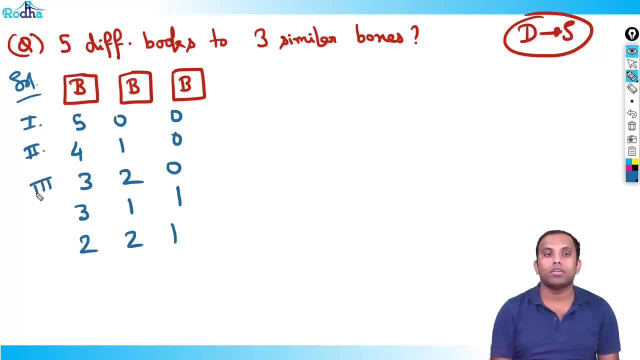 cases: first case, second case, third case, fourth case and fifth case. okay, now how many cases here? for there are five different books. let's say math, chemistry, physics, biophysics and hindi. also now, math, chemistry, physics, biophysics and hindi. also now, chemistry, biophysics, Hindi. there are five different books, right? so in first case five, all five can be. 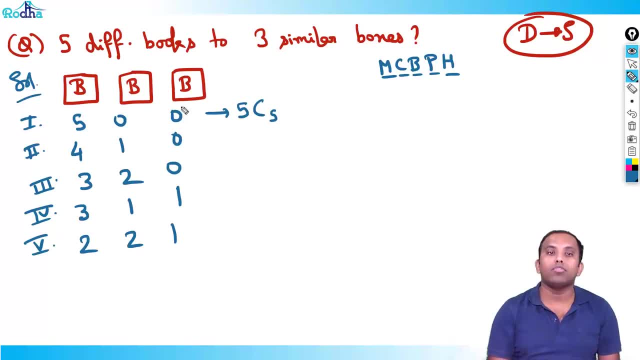 selected in one way, that is 5c5, and placed in any of these boxes, only in any of these boxes, in only one way. so 5c5 into one is only one. second case: 410 out of five books, any four can be selected in 5c4 ways. that means I can make 5c4 groups of 4, 4 books, and obviously now one will be every. 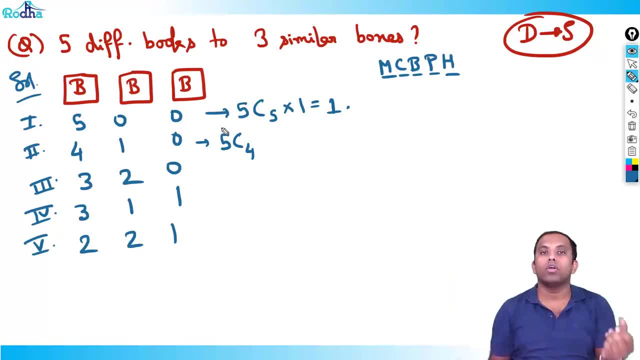 when you select any four book, one is left. so you have two groups now, one with four book, one with one, one book, right, there's two groups can be placed in any of the boxes in one way. so for making groups, only one way, for putting in boxes, only one way. right, that is fine, two groups, right. 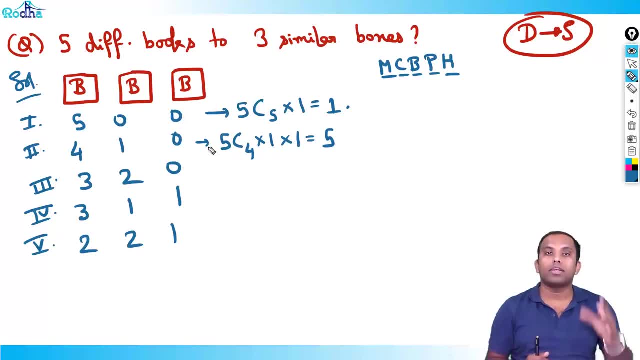 so only one way to put in the boxes: since you've selected four, so only one is left. only one is left right, so four and one. so you can't select it. so selection only one way: that book automatically is left, only one. after selecting four, three, two zero, three, two, zero. so 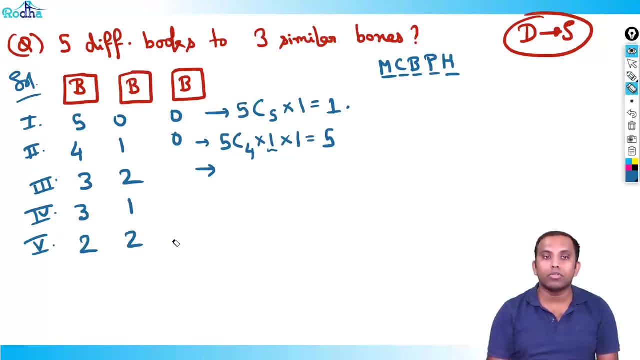 three, two, zero is what I think it is bit of. four, there's not in line here. we get a confusion here. three, two zero. three, one, one and two to one. okay, what is three, two zero here? three, two zero out of five books. selecting any three books in five. see three ways. okay, now two books are left, so two. 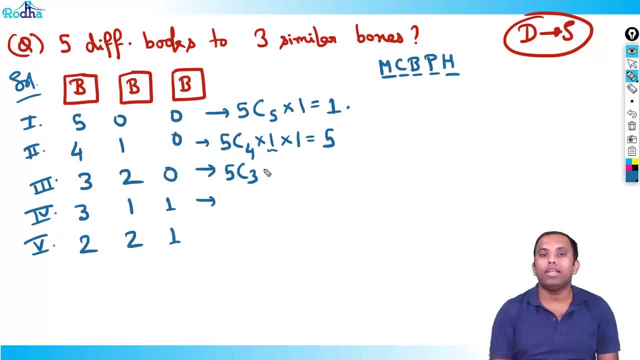 books are left and you select both. so only one way. right, you can write two c, two here, but it is only one way, okay. so out of five books, selecting any three books in five, see three ways. there are five, see three cases of three, three book. so when you select three book, automatically two are left out. 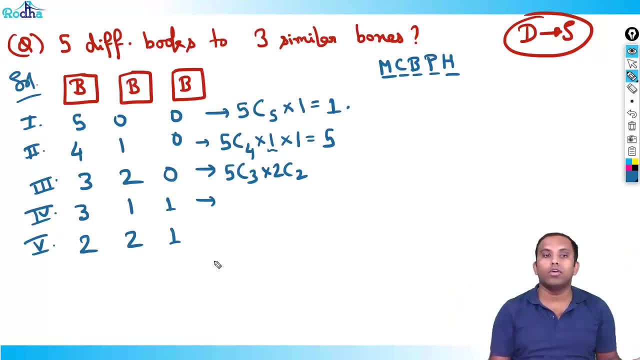 right, you have to select both the book now. so two c two. that is only one way, okay. so out of that, in one hand there are three books, in one hand there are two books. it's group of group of three. two you can place in any of the boxes only one way. 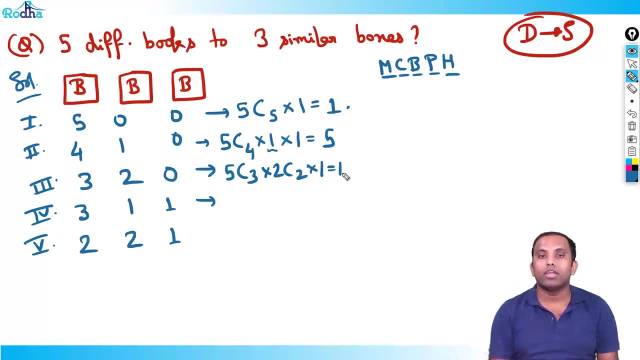 so five c. three is ten. so ten into one is ten. okay, three, one. one out of five books can select any three in five. see three ways: now there are two books left. okay, now there are two books left and you have to. there are two books left and you make a group of one one, so again, 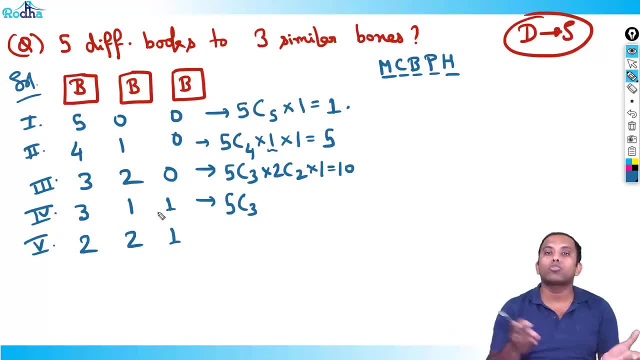 same thing. two books are left and you have to make two groups of one one. so absolutely no choice of making groups. one group will have to keep only one book right and shuffling will not do anything because those groups, when putting in identical boxes, only one way right. so that's why. 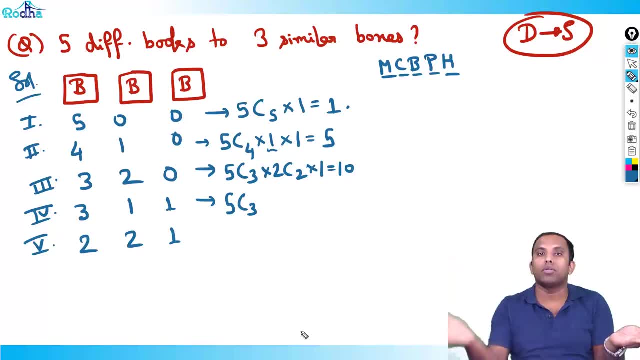 one group of three book, one group of one book and one group of one book. there are three groups right, putting all the three groups- that is three, one, one- in only one way, in any of the three boxes right, in all the three boxes: three, one, one, so only one way. so five c, three into one. 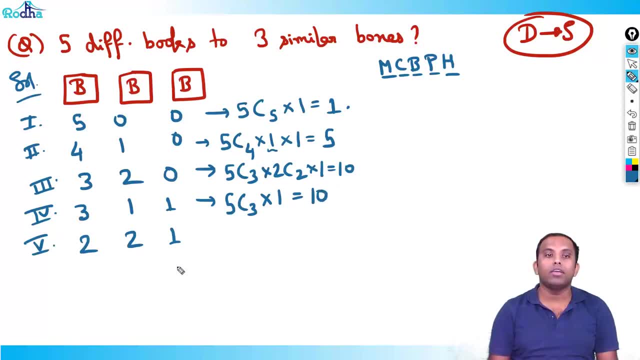 only, uh, this is only ten, this is ten, right, okay now. two to one, two to one, how many? for two to one here? see: for two to one out of five boxes. selecting any two boxes, sorry, out of five books. selecting any two books in five c two ways. okay, selecting two books in five c two is right now. now here three books are after selecting. 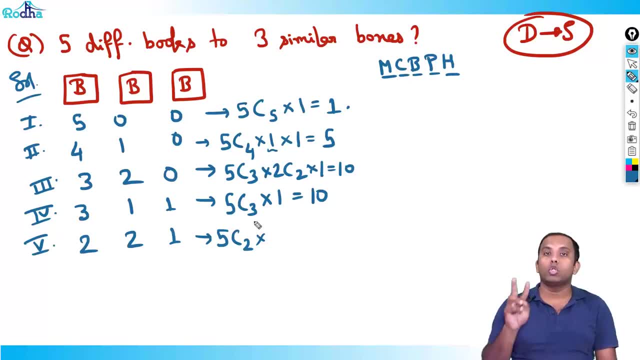 two books, three books are left. after selecting three books, two books are left right. so sorry, after selecting two books, three books are left Out of 3 books. you have to make 2 groups of 2 and 1 now. So again, the fight will come right. 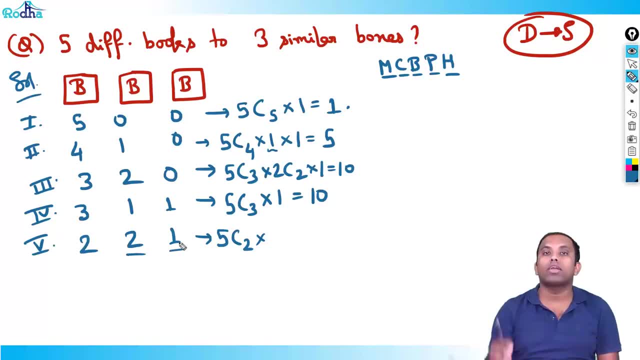 Now there are 3 books and you have to make 2 groups of 2 and 1. So again, which 2 will be there, right? So, out of 3 books, selecting any 2 books in 3-C-2 ways, right? 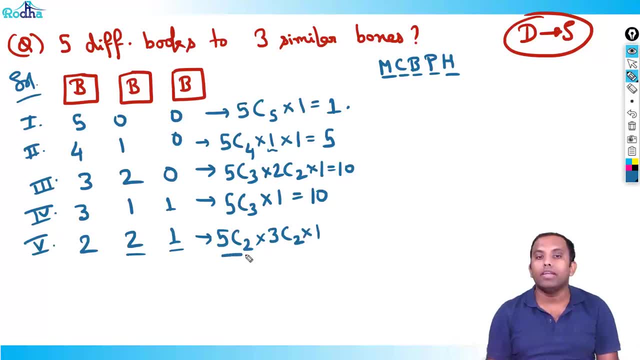 Now and only 1 book is left. so only 1.. Now, divide here by 2.. Divide here by 2.. Why dividing by 2? Same thing I told right: 2 and 2, repeating 2 times. you have to divide by 2.. 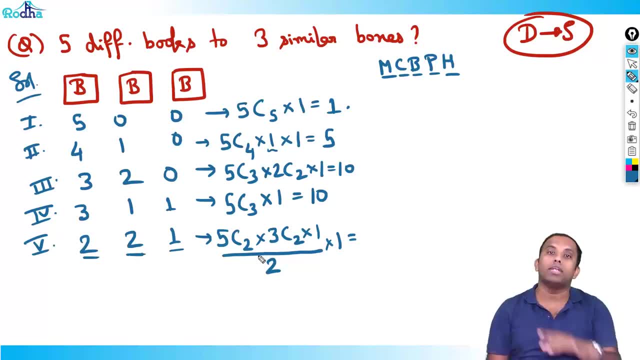 Any number other than 1, repeating twice, divide by 2.. Because there will be a symmetry. How will you find a symmetry? See, I'll tell you how to find a symmetry here. See if there are 3 books here. sorry, if there are 3 boxes here. 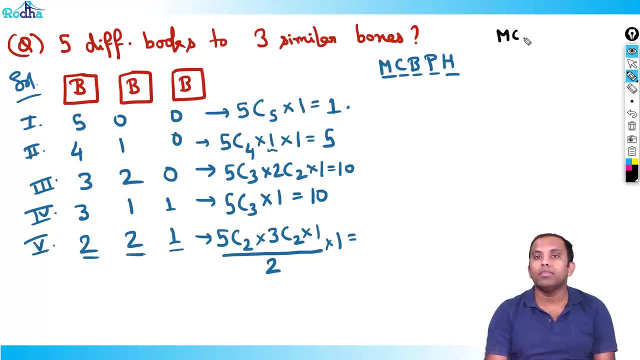 so 2 to 1, so let's say, 2 boxes are Maths, Chemistry, Biophysics and Hindi. right, Then you can change the data like Maths, Physics, Biochemistry and Hindi, like that. Okay, so a stage will reach. 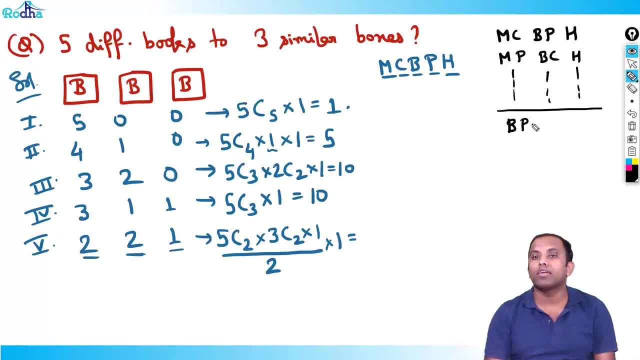 After that, the next will come as Biophysics, Maths, Chemistry and Hindi. Next will be Biochemistry, Maths, Chemistry and Hindi, right. So you see this, and this is same: Maths, Chemistry, Biophysics, Biophysics, Maths, Chemistry, right. 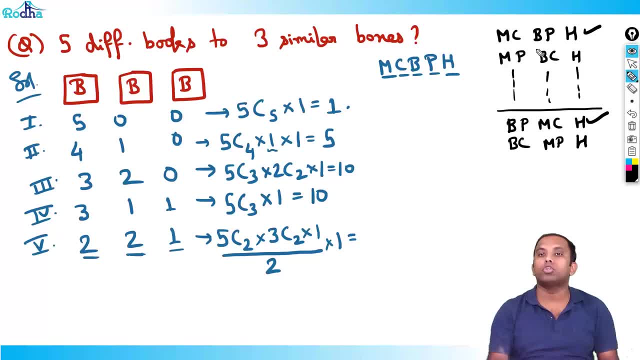 Hindi. So these two are same thing. because 2 to 1, right, This group of 2, 2 I can't differentiate because they have to be kept in identical boxes. right, This group of 2, 2 is same. 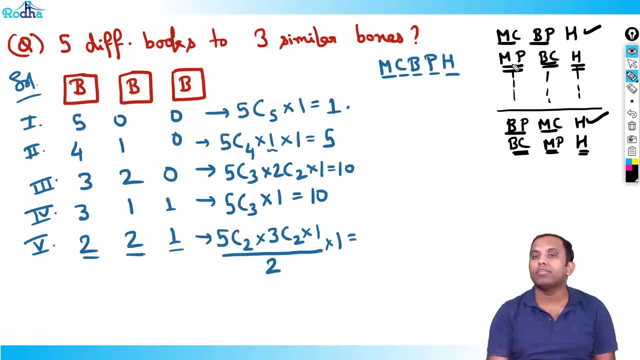 Similarly, this group of 2, 2 is same: Maths, Physics, Biochemistry and Hindi Biochemistry, Maths, Physics and Hindi right, So 2, 2.. What is in 2, 2 group: Maths, Physics and Biochemistry in both the groups right. 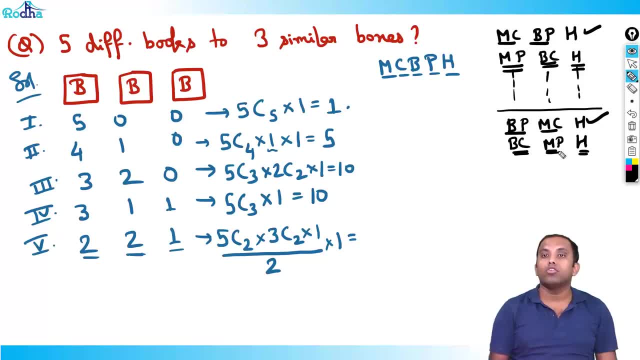 Order is not important because anyway, boxes are identical, right? That's why I told you there are always some symmetrical cases. So if you're trying to write 5C2, 5C2 into 3C2, there are 3 boxes. 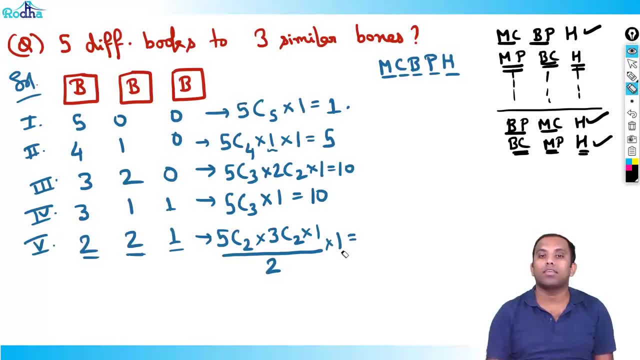 There are 30 cases, But there are not. there are not 30 cases, There are not 30 cases. There will be only 30 by 2, 15 cases. right, There are only 30 by 2, 15 cases. 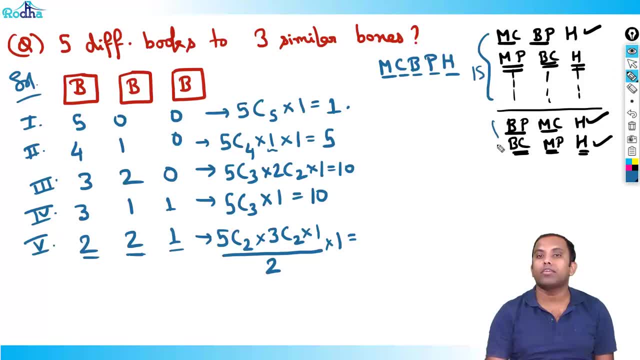 Because you see, first 15 will be same as last 15, right, You go on. So only 30 by 2, 15 cases will be here. Okay, so 15 cases here. So what is the answer for this question now? 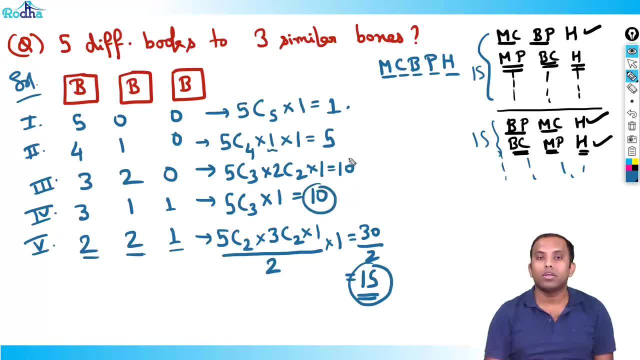 15 here, 10 here, Okay, 10 here, 15 plus 10,, 25 plus 10,, 35 plus 5, 40 plus 1, 41. So what is the answer? So answer for this question is what.